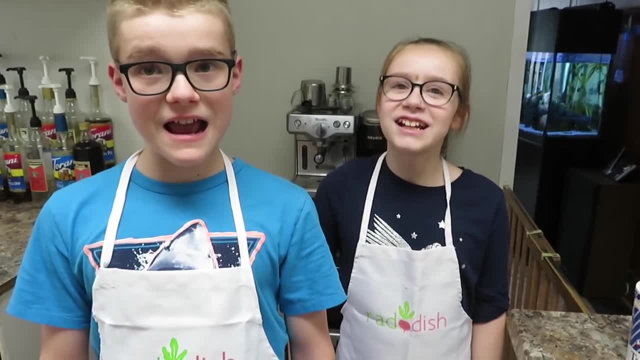 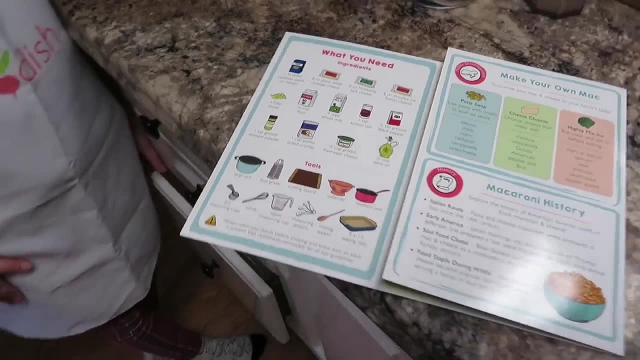 What are you two making for dinner? Baked macaroni and cheese. We love these recipes because they have pictures for us. Yep, Are they easy for you to follow? Yep, yep, Okay, so what are we going to do? first, Let's take a look. 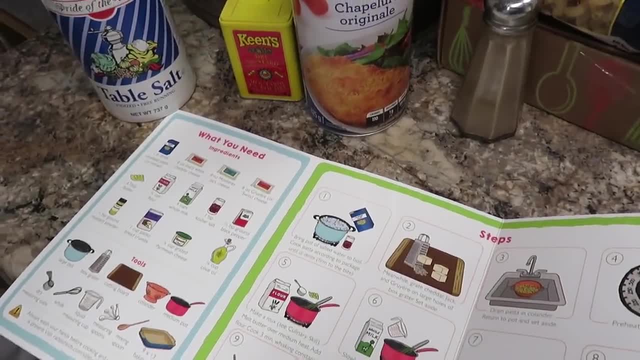 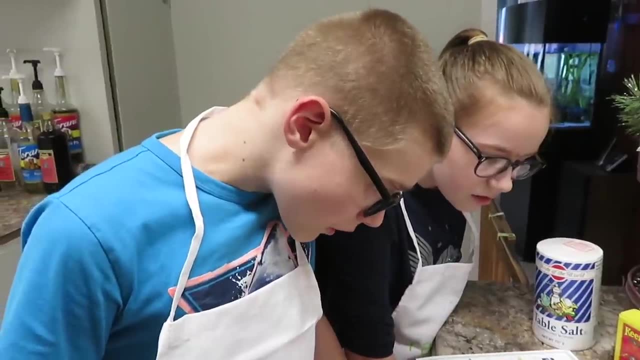 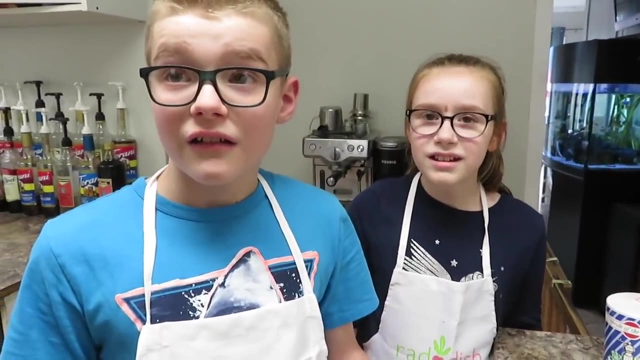 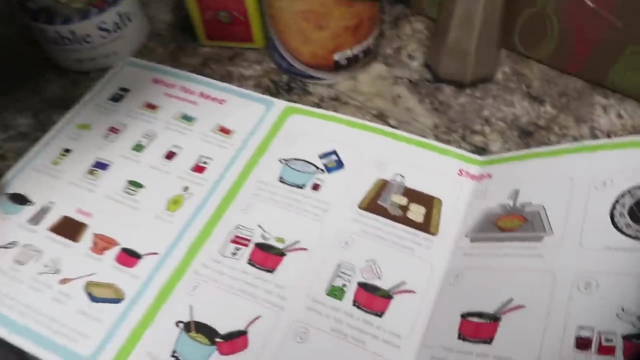 Bring part of salt water to Boil cooked pasta, according to package, until Al dente. Al dente, firm to the bite. So you guys are learning some new words as well, aren't you, Yep? Meanwhile, grate cheddar, jack and chlorella. 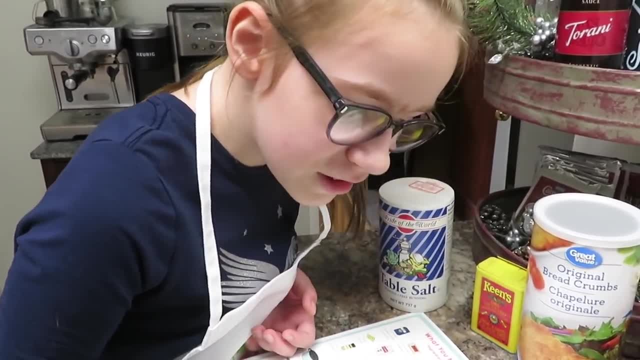 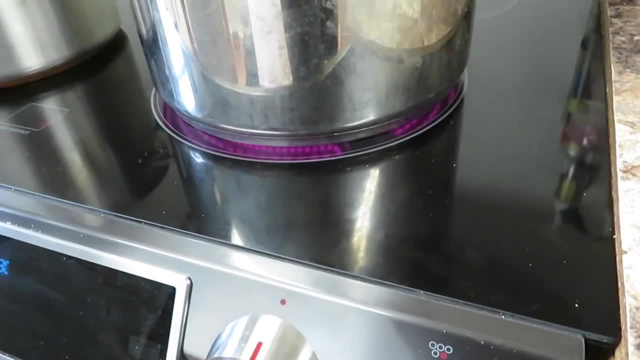 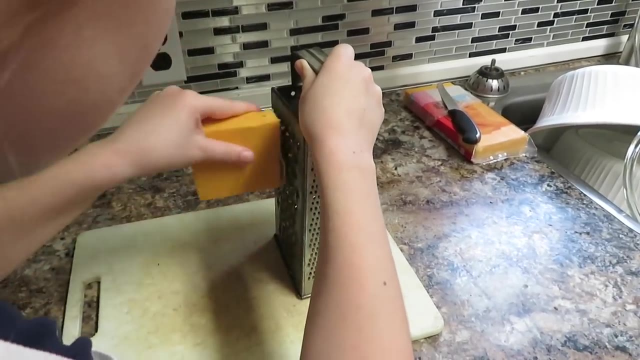 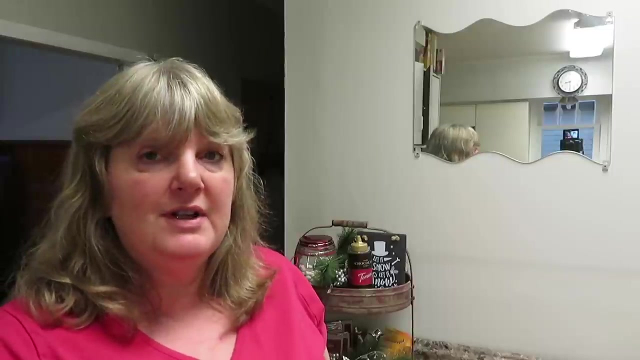 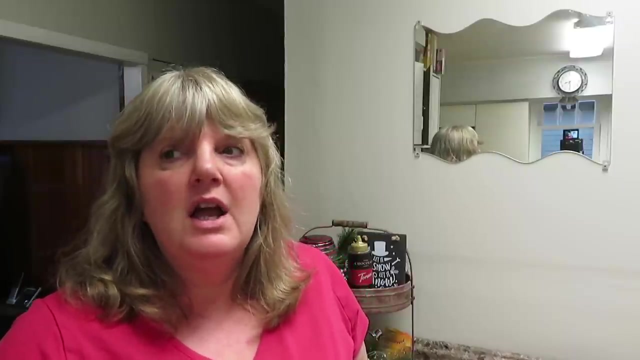 Eat, a large source of Grחka fishs side. I want to thank Radish Kids for sponsoring this video. We have been using the radish cooking program for the last three years, so when I'm cooking and when I'm jamming, you go to me in my face and say: 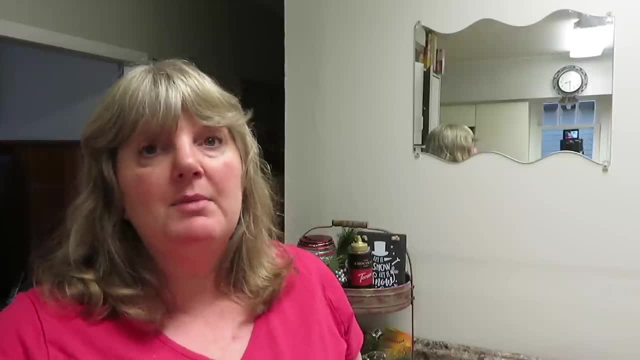 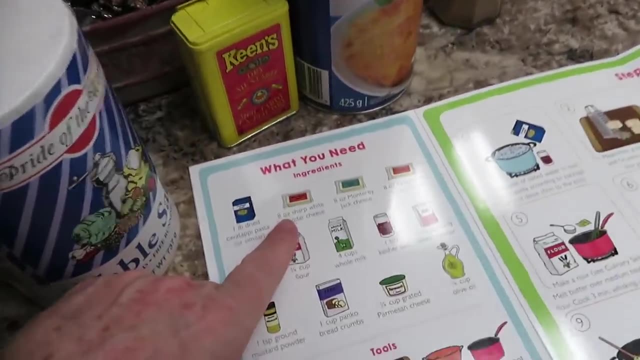 So when I'm saying that I think this is a great program, it's something that we've been using for the last three years without any sponsorship. So you're doubling this recipe and you need eight ounces of cheddar, eight ounces of Monterey. 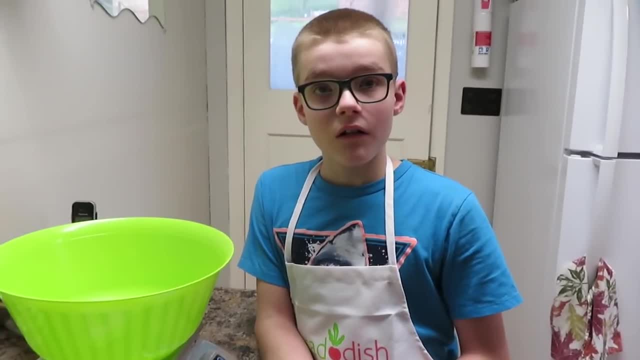 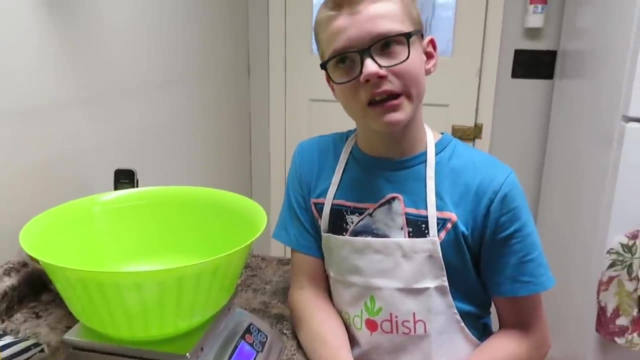 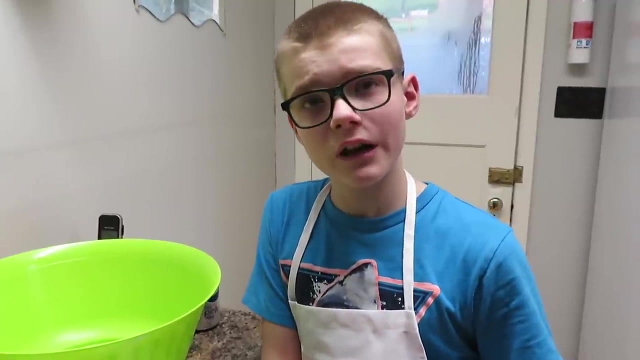 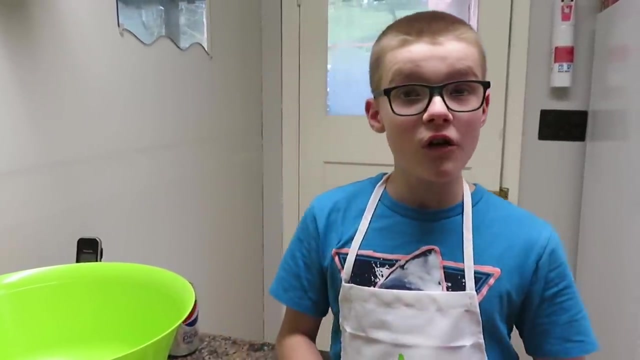 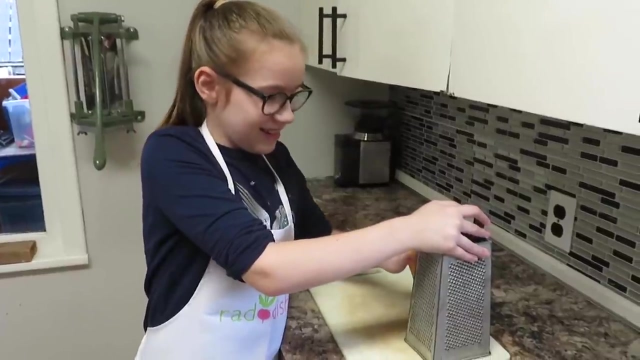 eight ounces of Swiss times two. So eight plus eight plus eight is sixteen, two, and four times two forty-eight. So we need forty-eight ounces of cheese. That's a lot Savannah, Yeah, Is grating cheese hard work, Yeah. 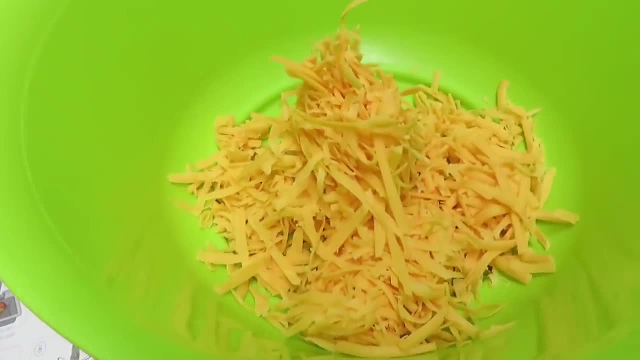 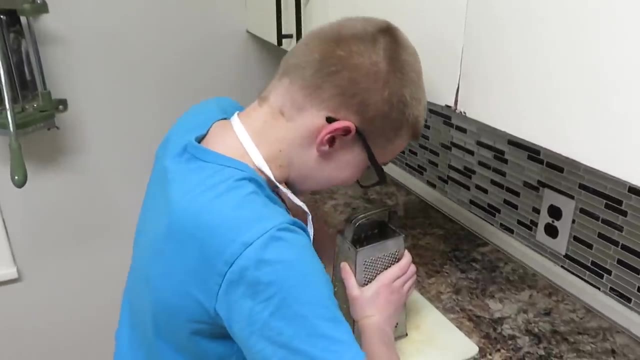 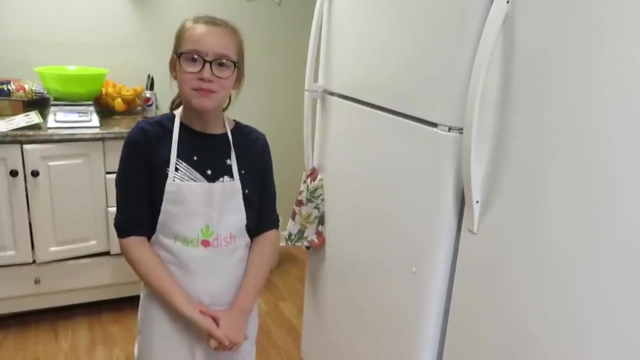 Okay, keep going. So you're faster than her at grating Yep, Are you sure? Yeah, What do you think? Is he Nope? Is that why we're waiting for him? Mm-hmm, What is the best thing about the radish recipes? 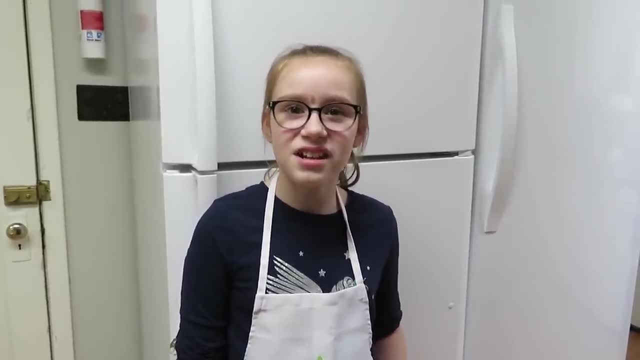 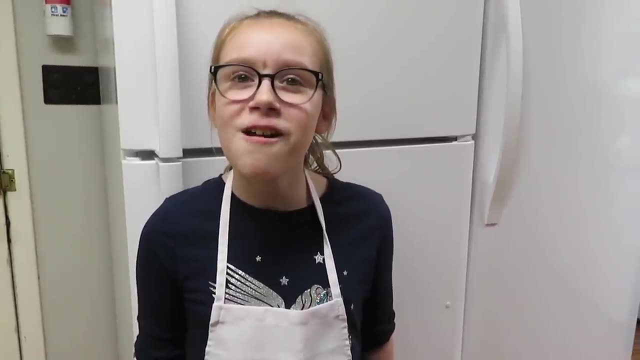 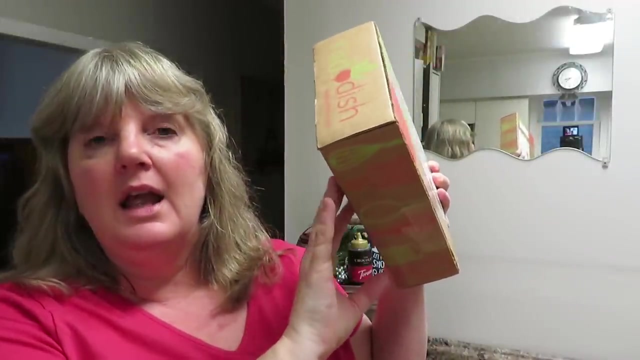 There's pictures that you can understand. So it helps you understand the writing with the pictures. Yep, I really like these pictures because I can almost do it by myself. So the radish program comes in a little box like this. It comes once a month in the mail and it's a subscription service. 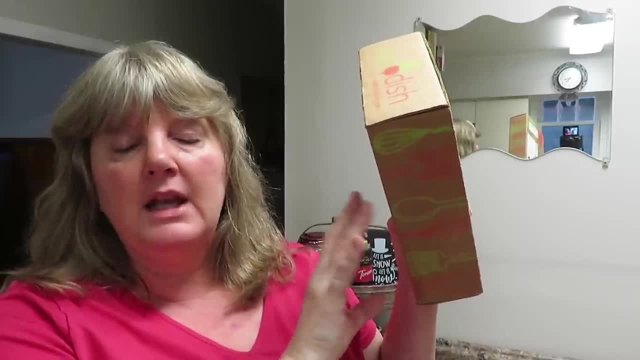 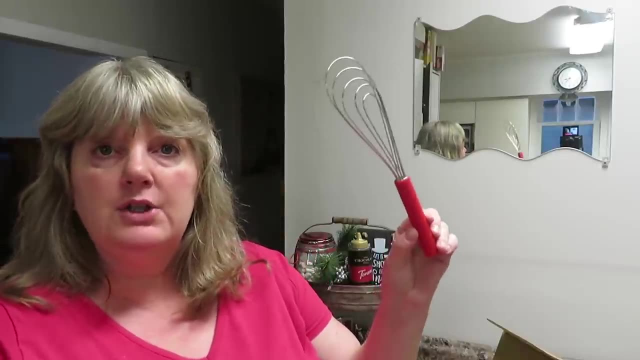 It's not a food service. No food comes in the box. It's just recipes that the kids can make each month. When you get the box each month, it comes with a kitchen utensil. This month it's a flat whisk. All the utensils come in a box. 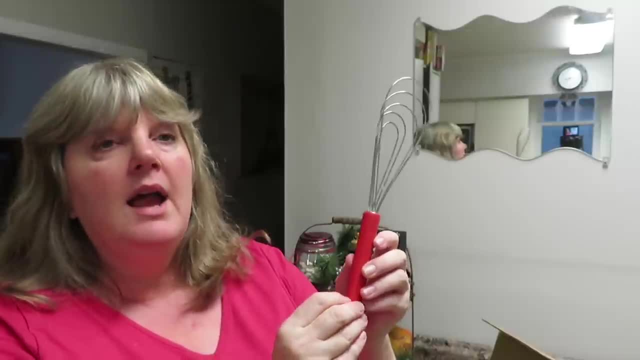 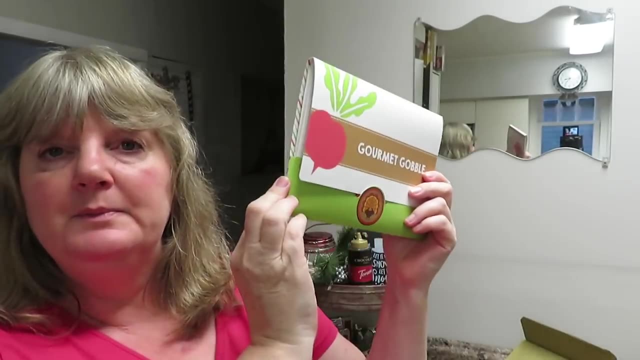 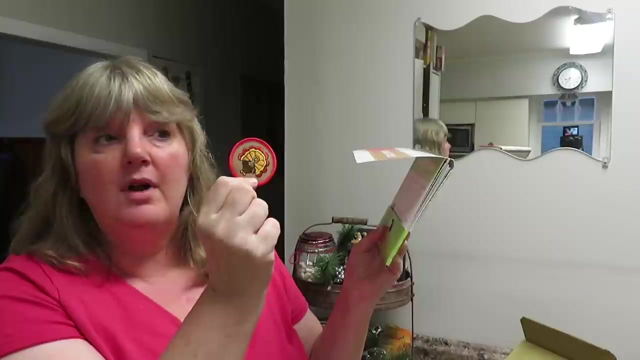 All the utensils have been really good quality and the kids are building up an amazing supply of kitchen utensils. The recipes come in this nice little file folder. This month is gourmet gobble. When you open it up it comes with a little patch that can be ironed onto their apron. 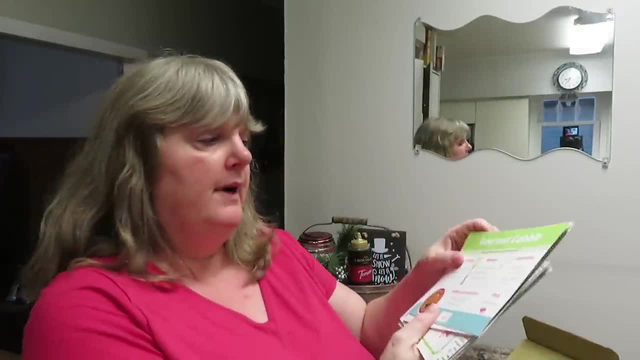 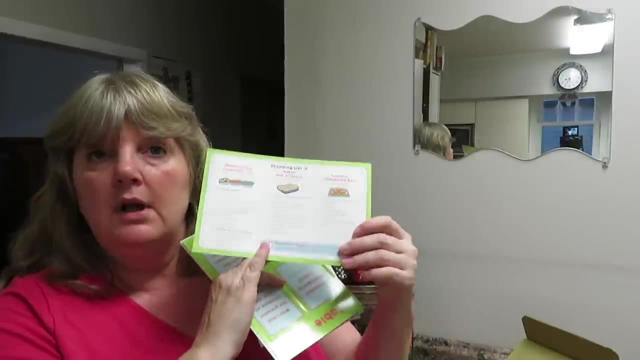 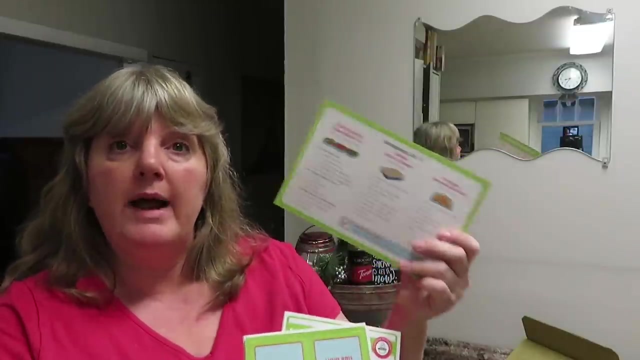 once they've completed it, When you open up the file folder, you get a shopping list, which is ideal. We will take these shopping lists. The kids will go through and see what we have at home and then they'll take this card to the grocery store and we will practice their life skills, learning how to shop based. 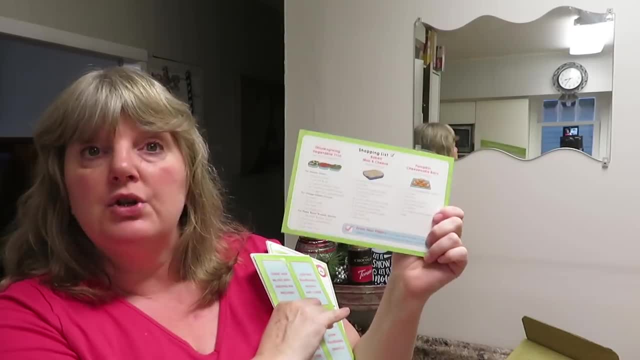 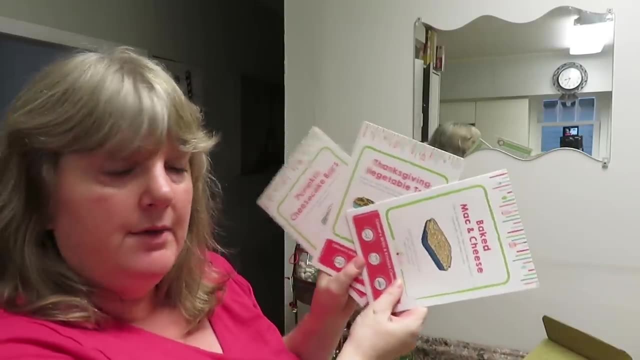 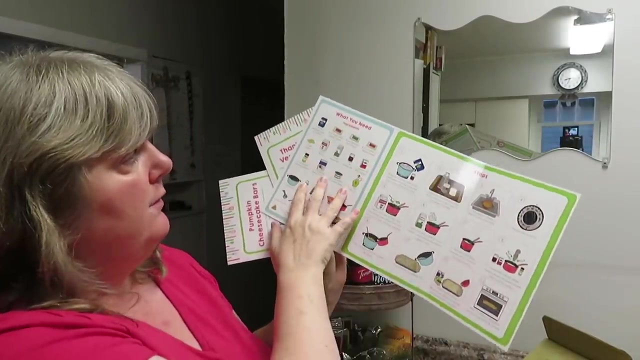 on this, following through and making sure that they have all the ingredients before they start. You'll get three recipes every month and they are plastic laminated. They open up and they have visuals here: Visuals of what ingredients you need, Visuals of what tools and visuals on the step by step directions. 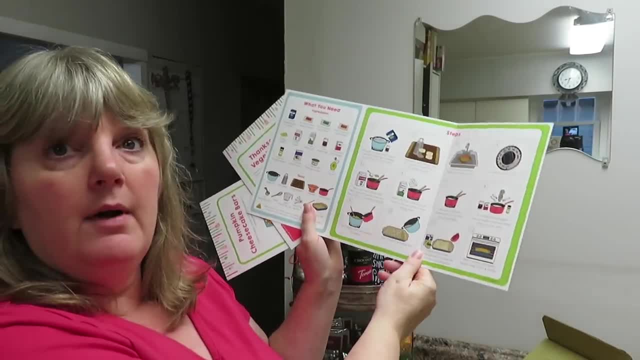 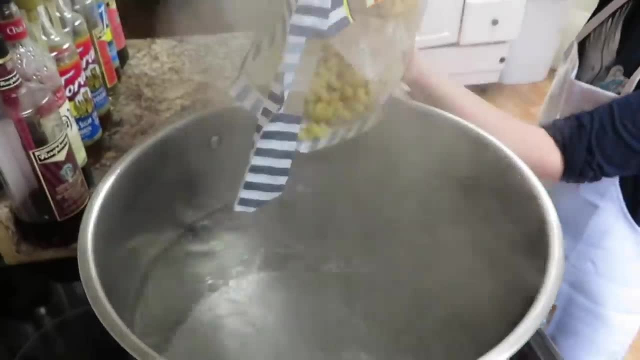 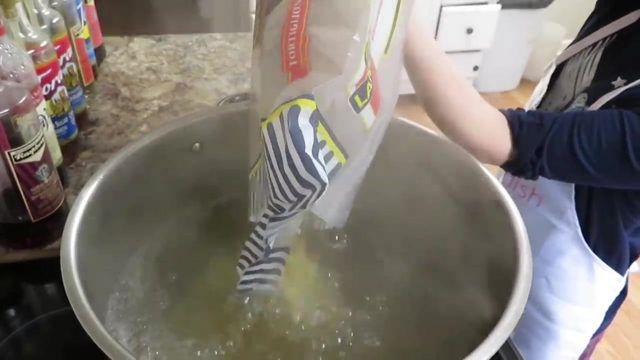 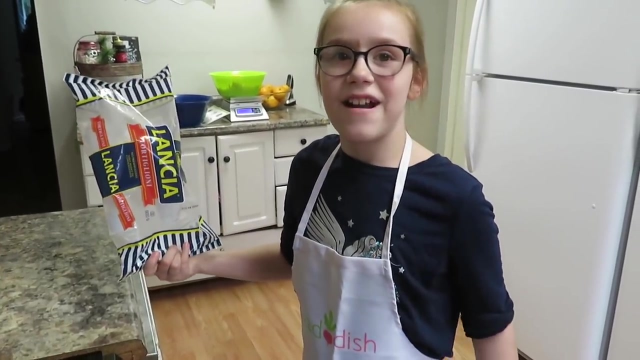 There's written words and pictures to help with the kids that aren't quite at a reading level where they can follow the instructions. And what was the special word it said for how much it has to cook? Do you remember? No, So, Jacob, do you remember the word that it says? 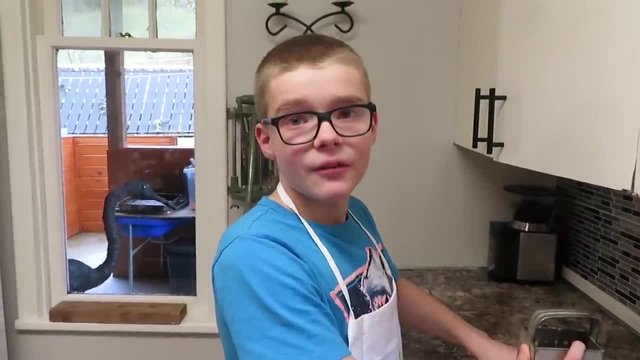 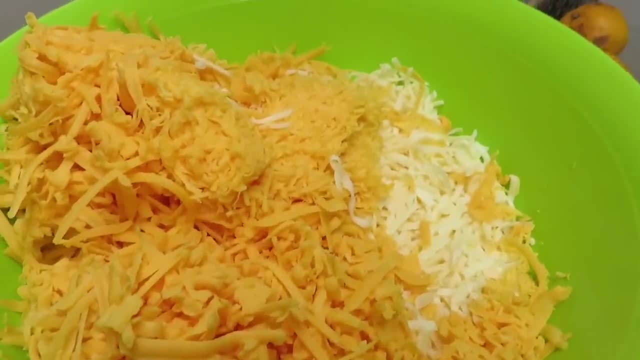 How much to cook Odonti, And that means that it's firm to bite. One thing I like about these recipes is it gives you substitutions, So we don't have all the cheese that it had suggested, but it tells you different types. 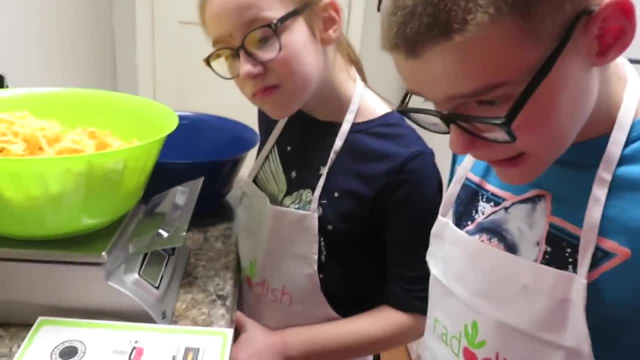 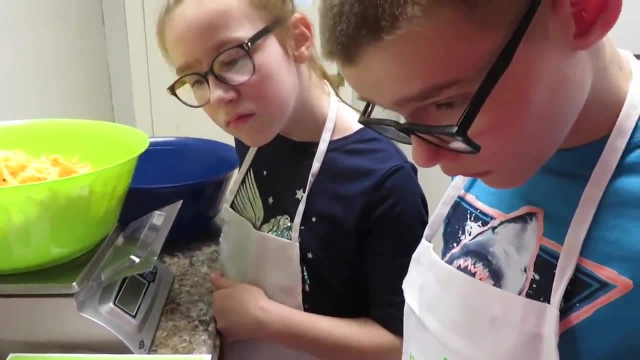 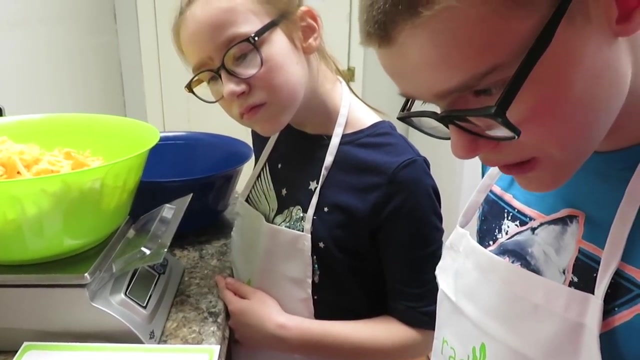 that you can use that we had on hand. Make a roux, Make a roux, Make a roux. So that's our culinary term that we're learning this time. Melt butter over medium heat, Add flour, Cook three minutes with constantly. 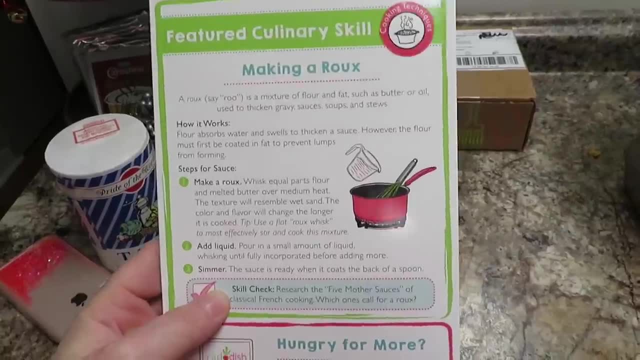 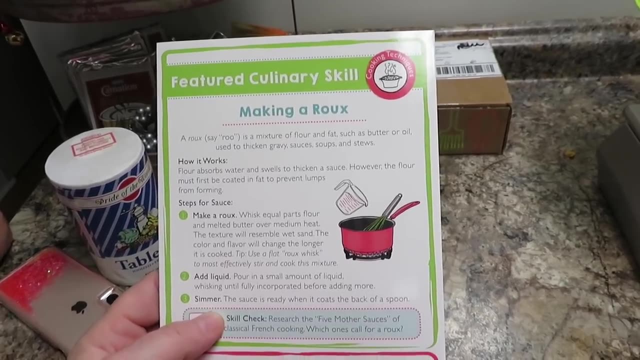 I really like the fact that they're teaching them the culinary skills, so when they move on to other recipes, they have learned a lot of the basics, even things that a lot of adults haven't learned how to do yet. Okay, so we're going to need a whisk. 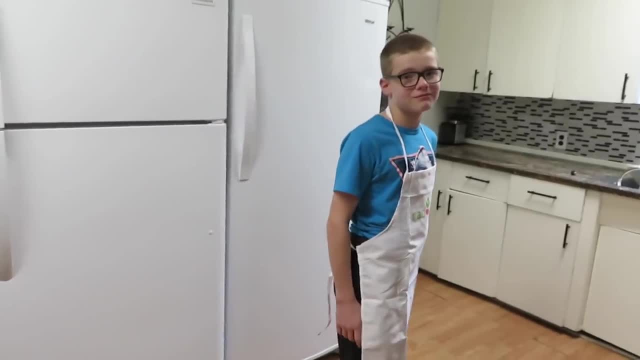 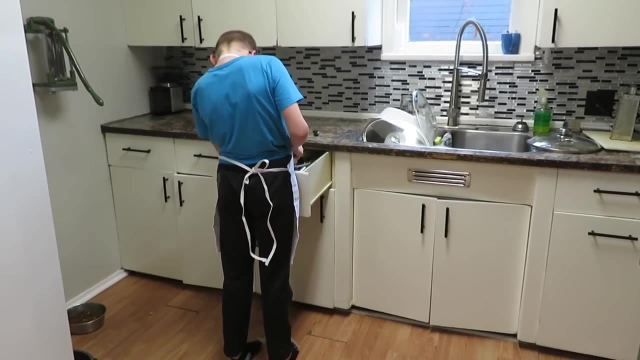 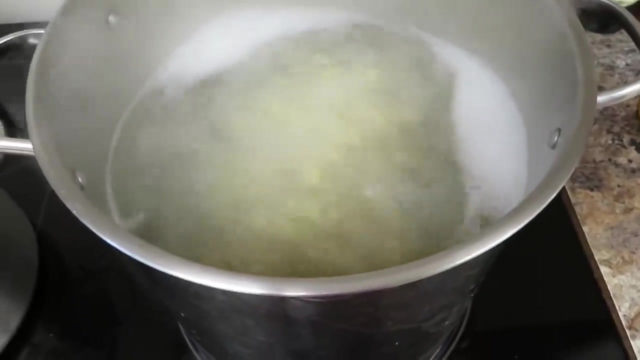 Do you know what a whisk is? No, Yep, Get us one. A whisk is this: Savannah, your noodles are boiling now, So we're going to have to pay attention, because that means they're going to be odonti soon. 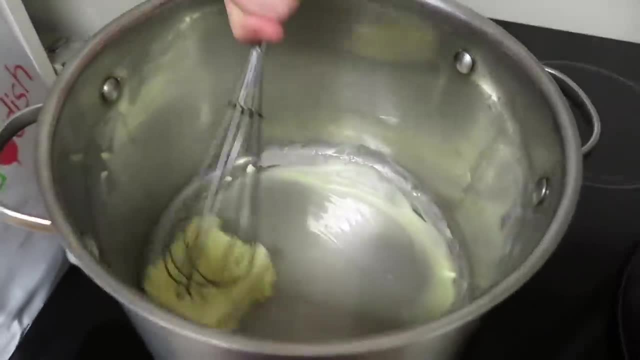 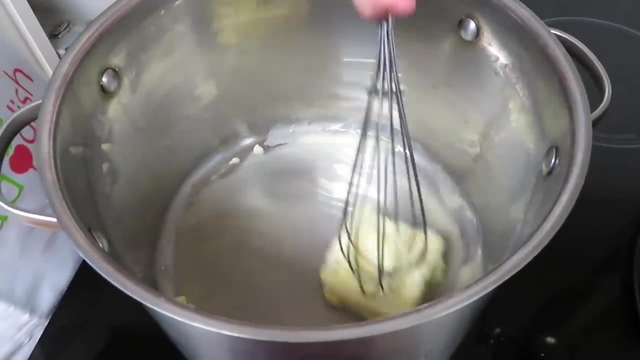 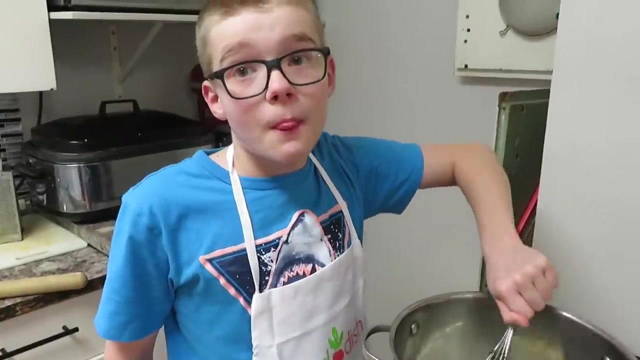 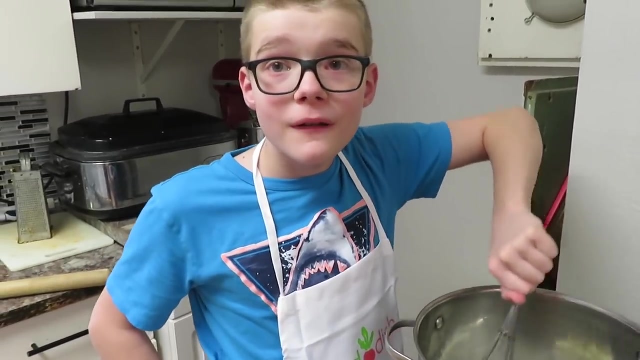 Look at the pop. Oh, your butter's starting to melt, Yep. And once it melts, you have to add the. What are you going to Sugar? We're not adding sugar, We're adding flour, Flour. So when you mix butter and flour together, it makes it so that it's a thickening agent. 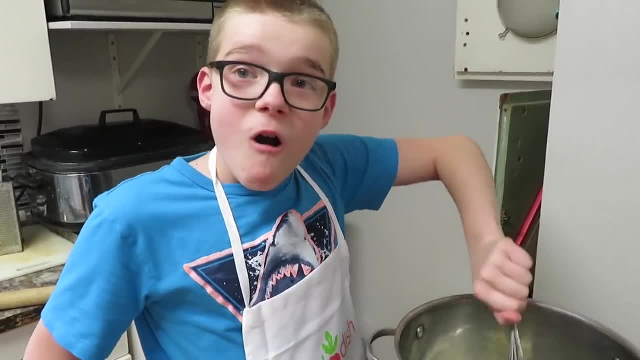 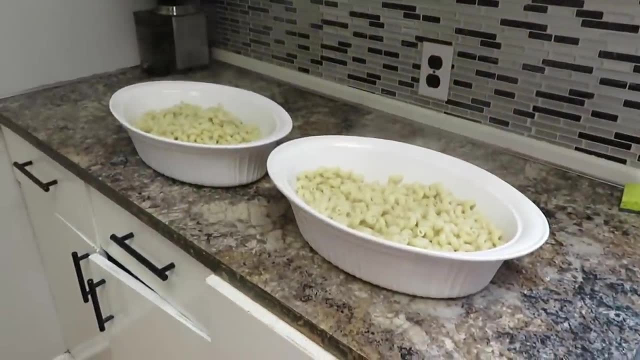 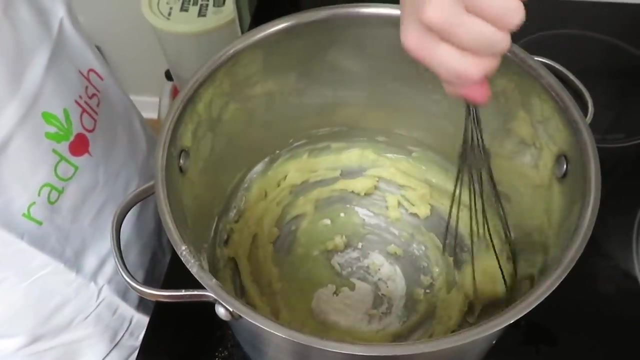 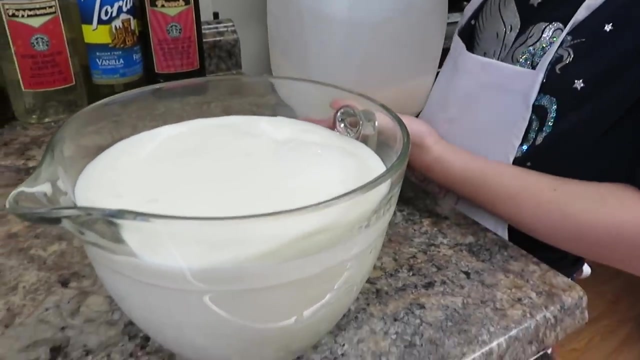 So it'll make your cheese sauce thicker. It's all mixed in. Yeah, Yep, Good, Nice. How much milk did you need? Eight cups, Eight cups Whoa. So we added a little bit of milk. Got to get it all mixed in really well. 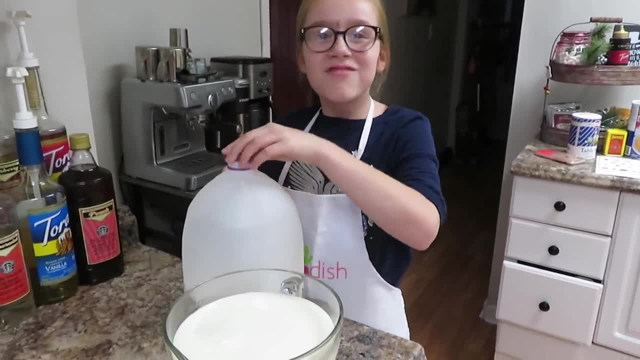 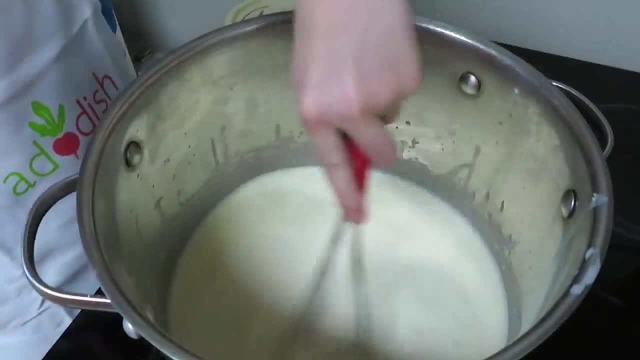 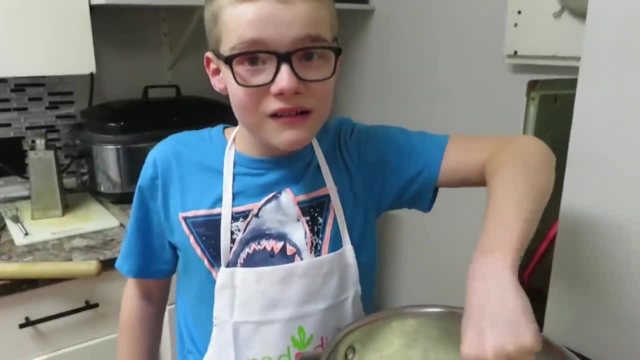 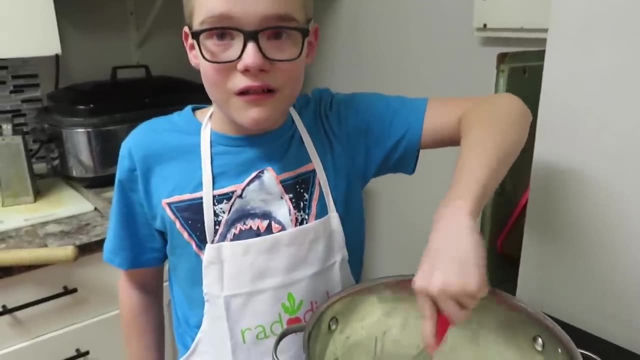 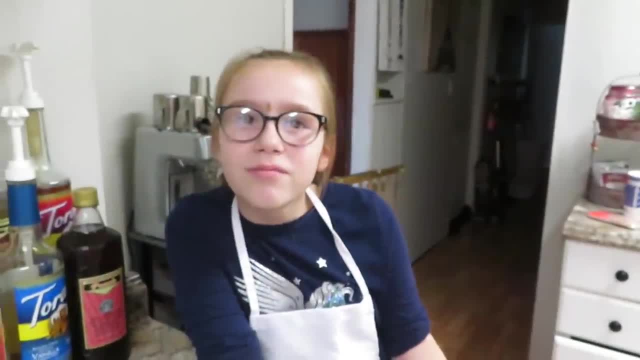 dish where you want to have a thickened sauce, so maybe soup, you could do it with this method. What would you make using this method? Mac and cheese and gravy. Mac and cheese and gravy- That's what you would use it for. 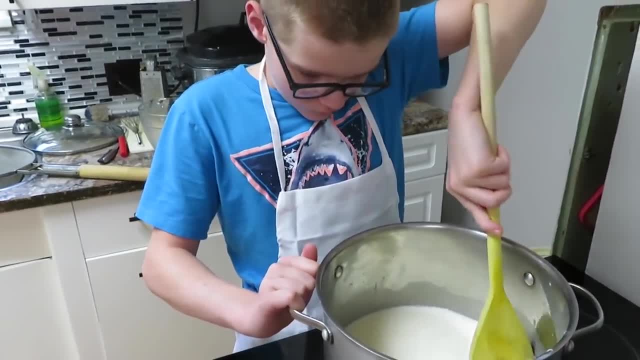 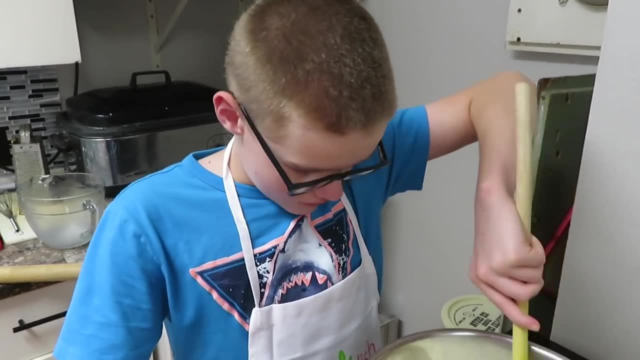 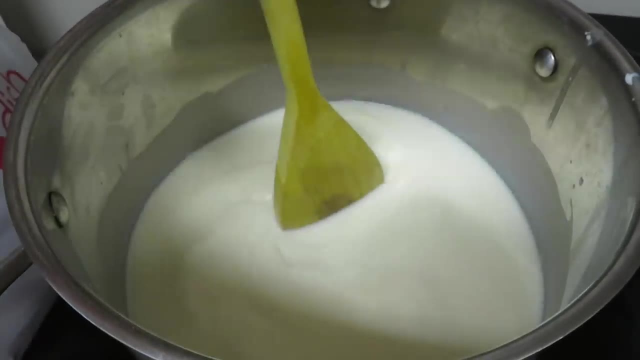 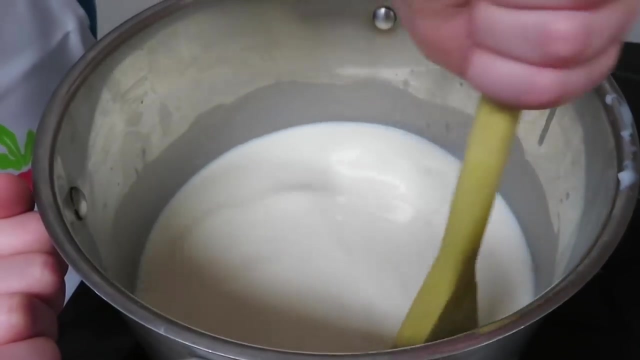 Yep. So we're going to keep stirring this slowly And we're going to know it's ready when it coats the back of the spoon, so that when take the spoon out there's still sauce on there and we need to stir it calmly so we're not making waves or splashes, because if it splashed on us that would. 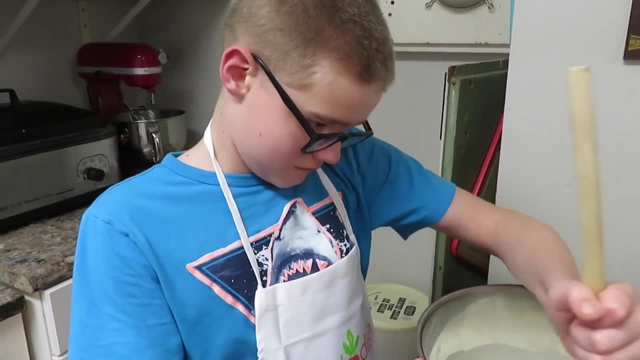 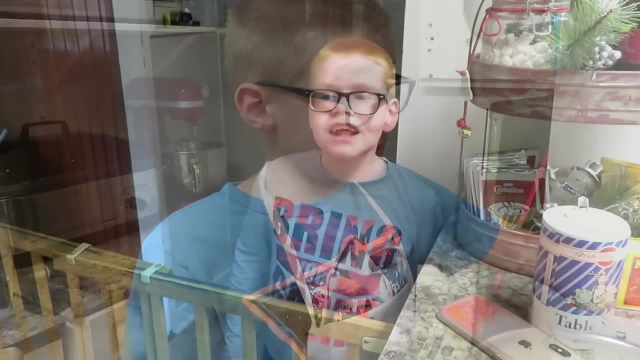 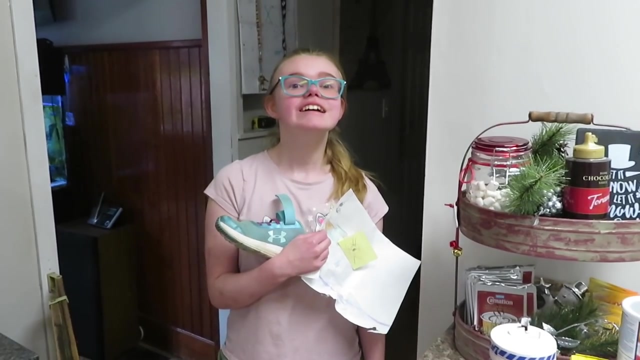 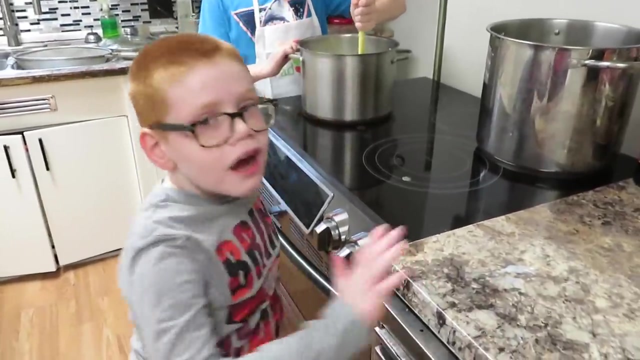 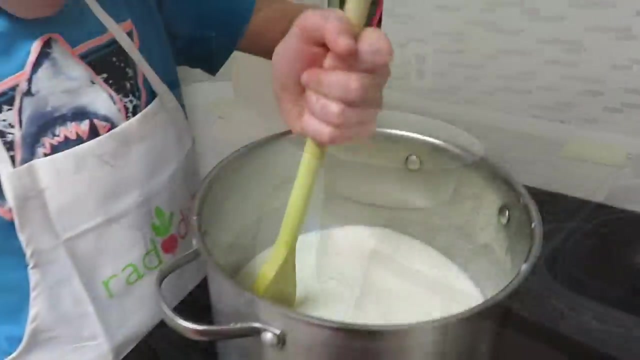 hurt because it would burn us. yeah, and I might cry really, really loud. yep, do you think they're good cooks? yeah, smells delicious, it's hot there and please be careful. yeah, I know that one's empty and you see it starting to stick on the sides. 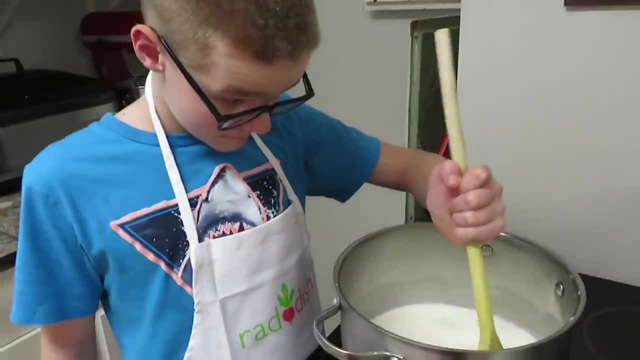 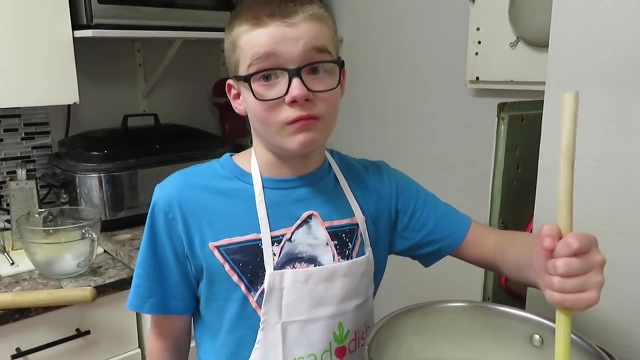 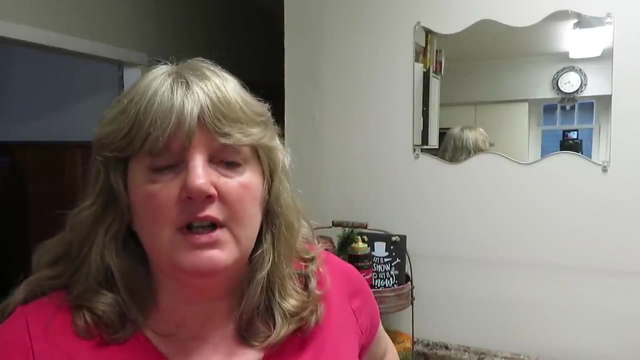 a little bit. yeah, okay, so that means it's getting closer, but we don't want to rush it, otherwise it won't thicken up and we'll have macaroni soup, yeah, so Radish is having an amazing Black Friday sale. so if you're interested, if you are buying a, 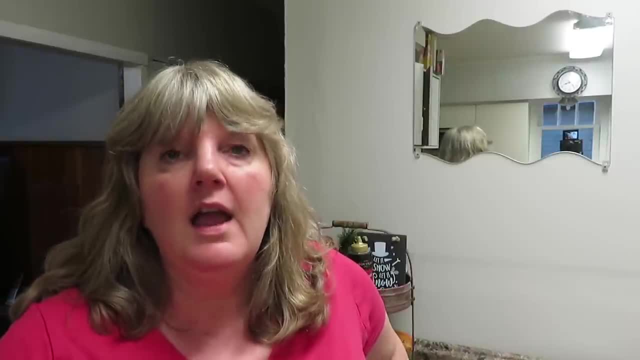 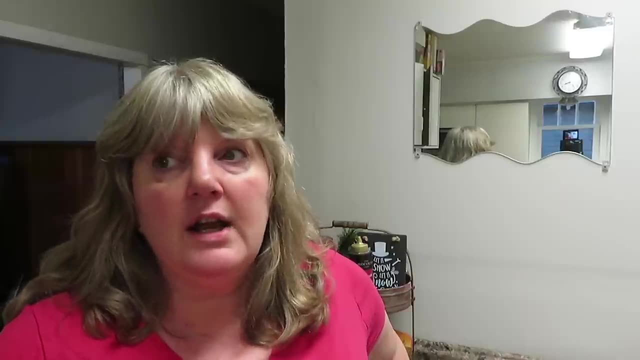 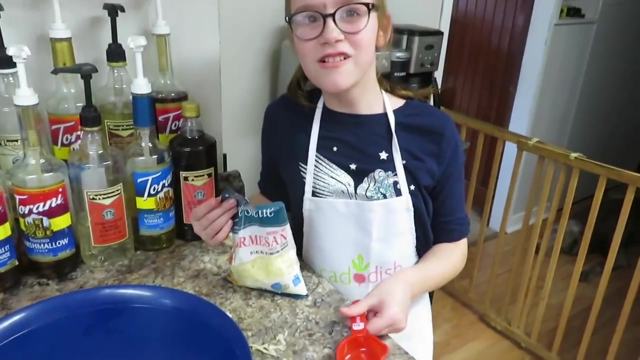 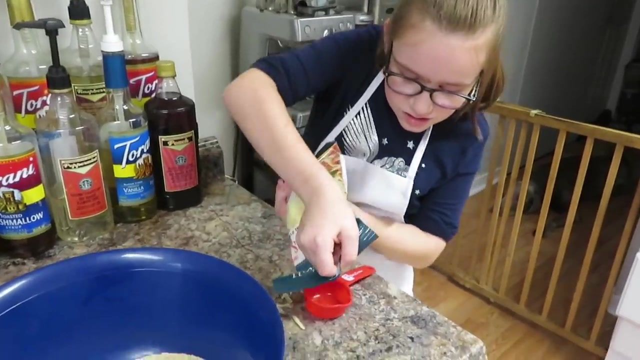 six-month subscription, you will get one month for free, and if you buy a 12 month subscription, you're gonna get two months for free. so if you're interested, check out the link in my description. is this good? I don't think you quite filled that up. hmm, what do you think? yeah, well, if we don't measure. 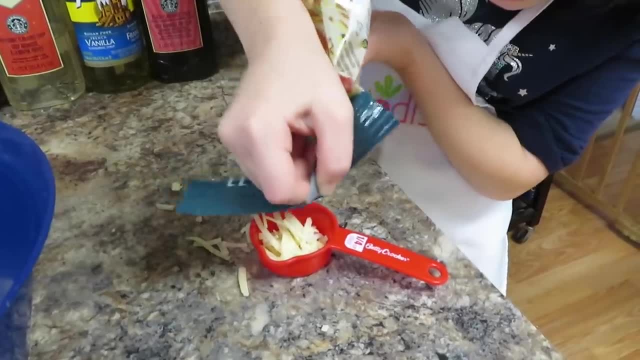 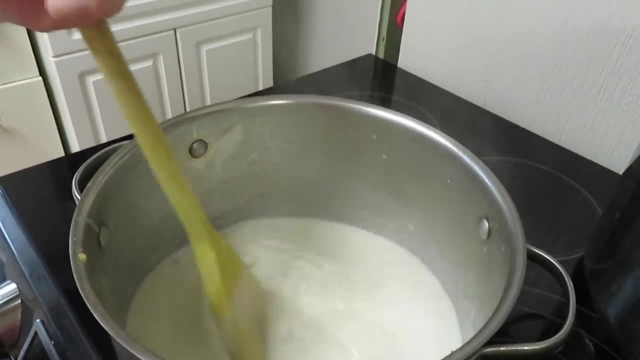 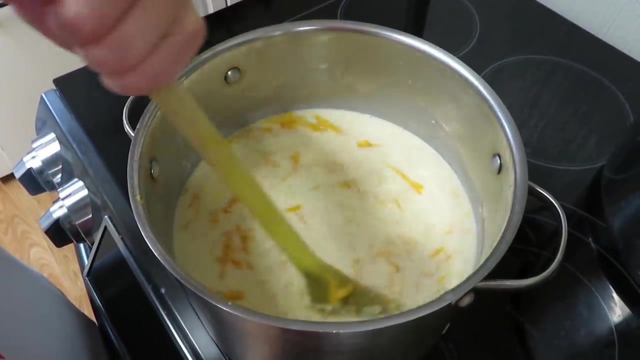 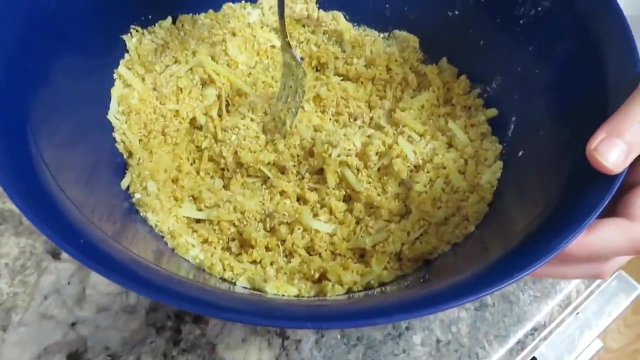 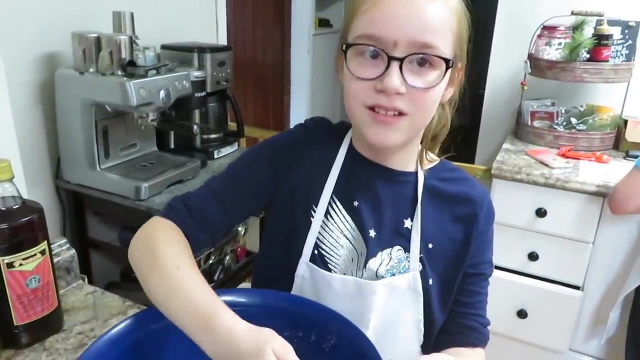 properly, then that affects our recipe and it doesn't turn out right. next, we need to melt the cheese in here, okay, okay, so I'm gonna put in a bit at a time. you're gonna keep stirring foreign, foreign bread and breadcrumbs. yeah, this is going to be the topping for your macaroni and cheese, okay, do. 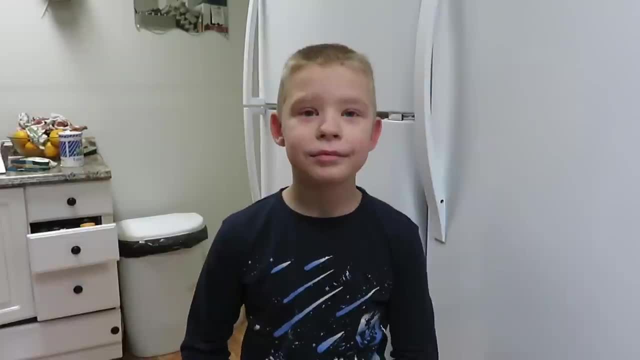 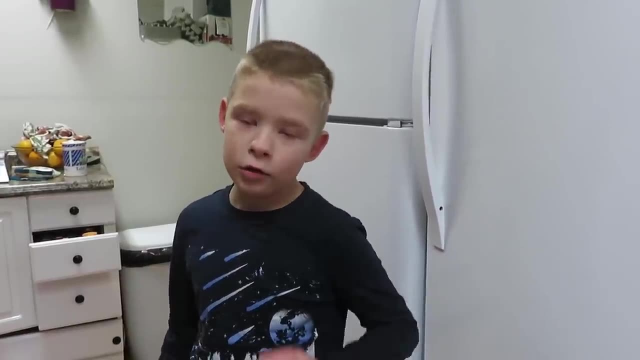 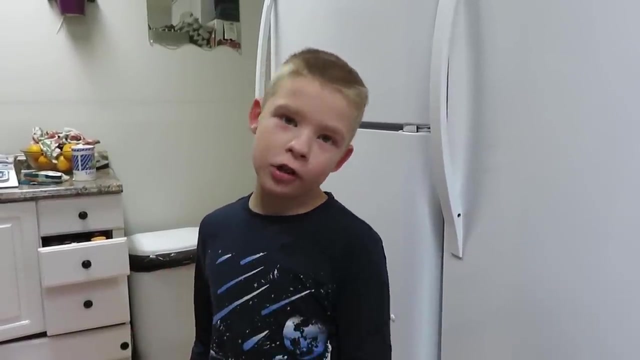 you like cooking with radish recipes. yeah, why do you like to cook with radish recipes? because it's like fun to do. it's just it's. it's just really nice to to, to make dinner for, for, for, for, for, for, for people that don't want to make dinner. that's true, it's really nice when you make dinner and I don't have to. 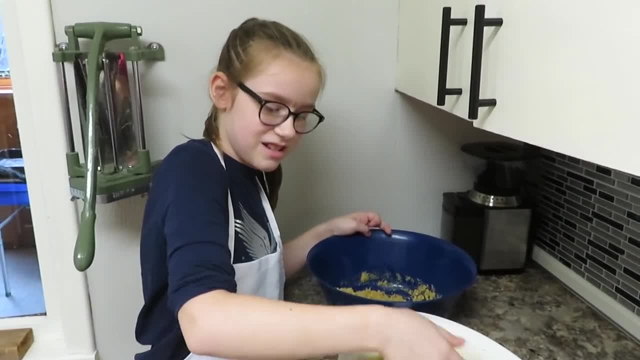 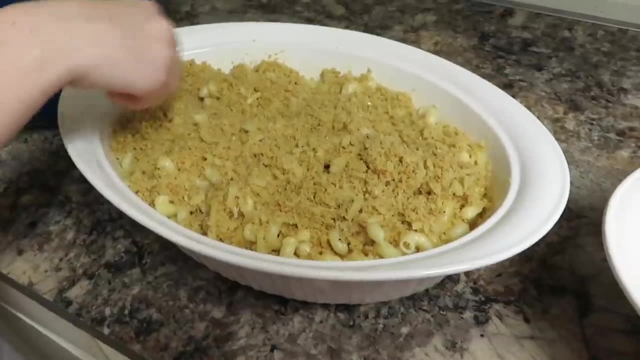 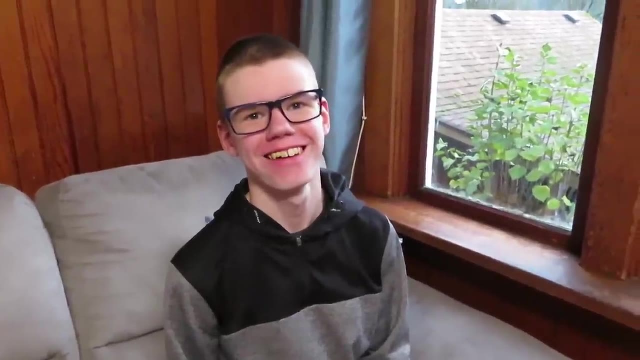 looks delicious, Savannah, yeah, do you think it's ready for the oven? yep, I can't wait for dinner. so, Dean, did you have to fight the girls off at the store with your new glasses because you look so good? no, well, isn't that what you thought? yeah, that all the girls were going to be after you. 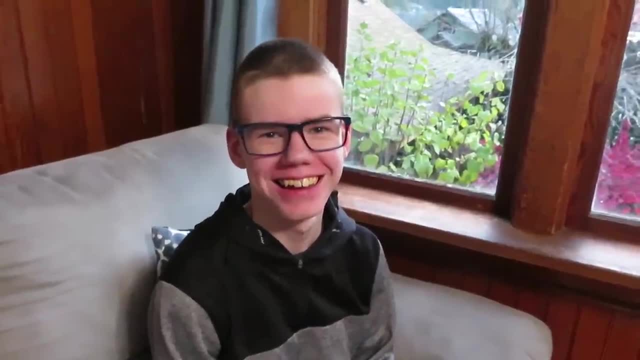 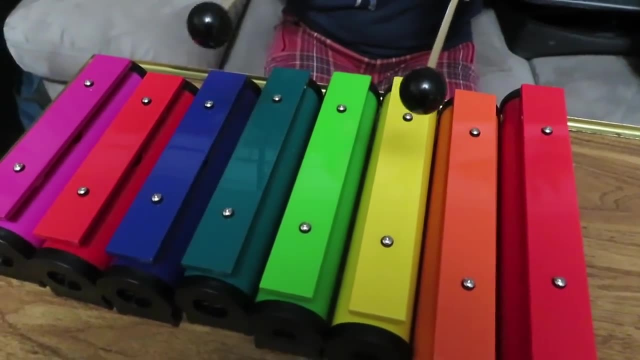 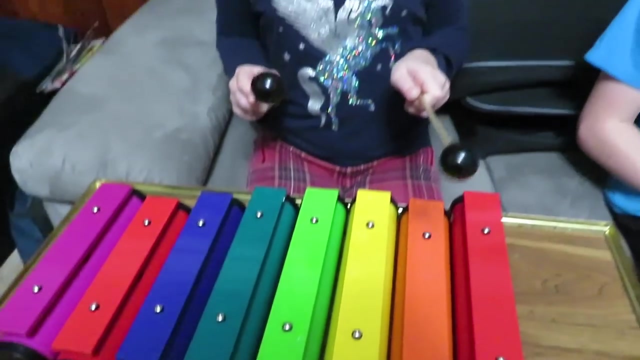 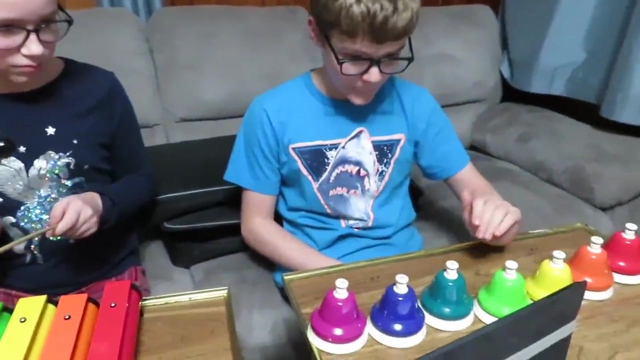 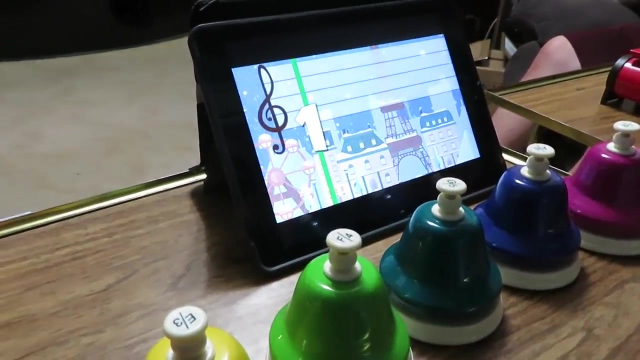 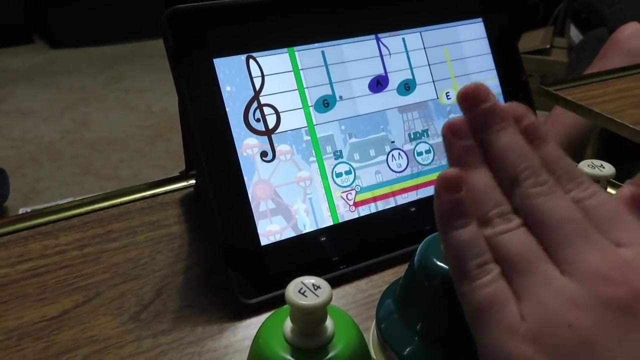 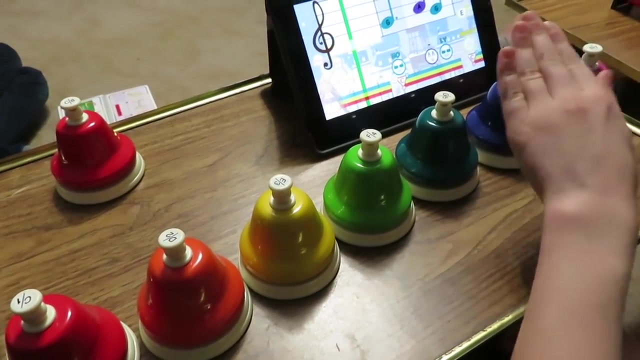 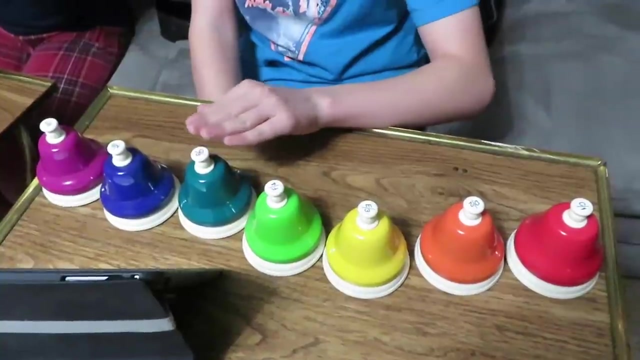 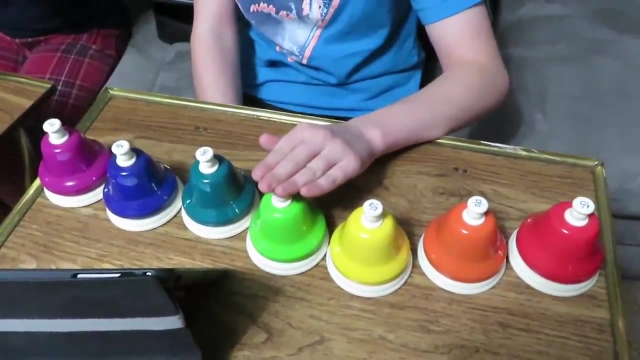 has it been hard going outside? have they been chasing you? no, not yet, not yet, okay. foreign foreign foreign foreign Holland foreign foreign foreign. so foreign foreign foreign. thank you, Thank you. bye, bye, Have a nice day. Have a nice day, Have a nice day, Bye, wer-youngly. 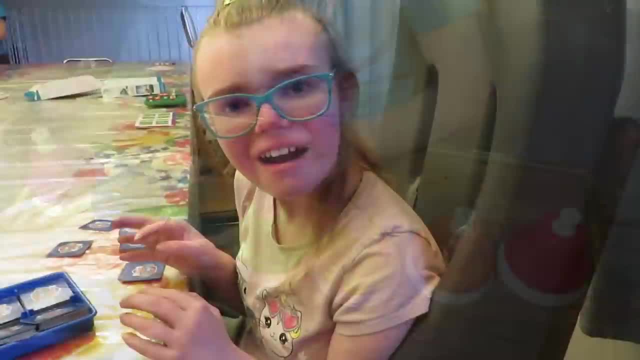 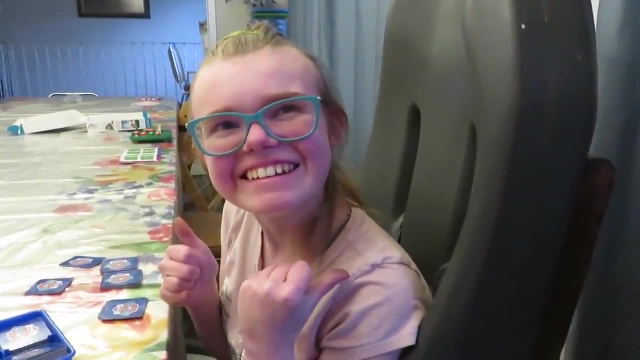 In the middle of your bed. Happy Sunday, Happy Sunday. So, Laura, what do you think of your new glasses? Good, I think they look really good And I really like the color of them. You actually got two pairs, didn't you? Yeah?